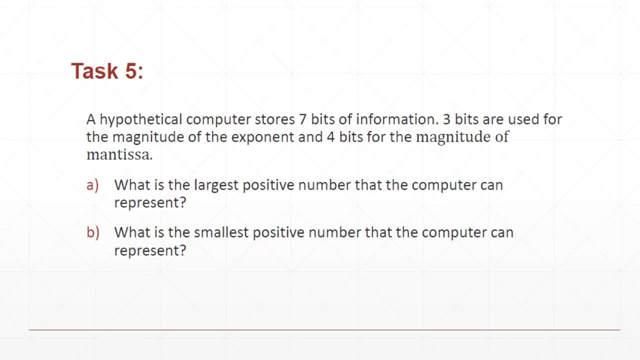 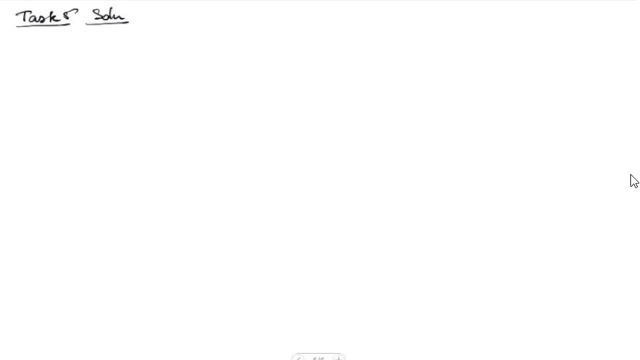 So let's start working on this now. Let me write little bit details again. So we have 4, 3 bits for exponent and 4 bits for magnitude. sorry, mantissa. Okay, now we need to find out for A, the largest number that the computer can represent. 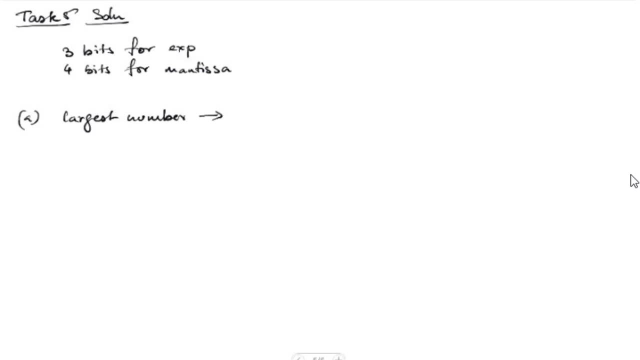 So the largest number will be always any number in binary. we start with 1 point Here for us in the floating pointer presentation, so we always have it with 1 point at the beginning, And then we have got 4 bits for the mantissa, so we'll have to fill up 4 positions here. 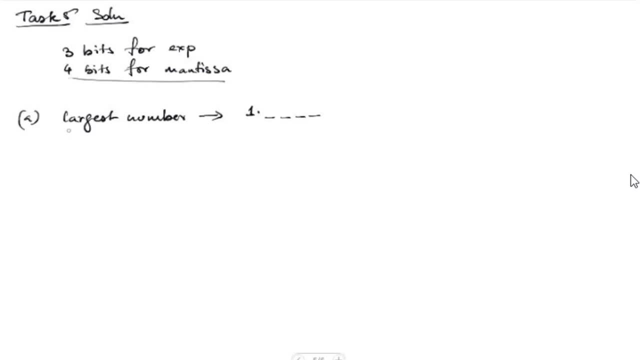 But then we need to find out the largest number that's possible. So we'll fill up for us like the largest number would be something of 4. Of course, which is all 1s in the binary system, right? 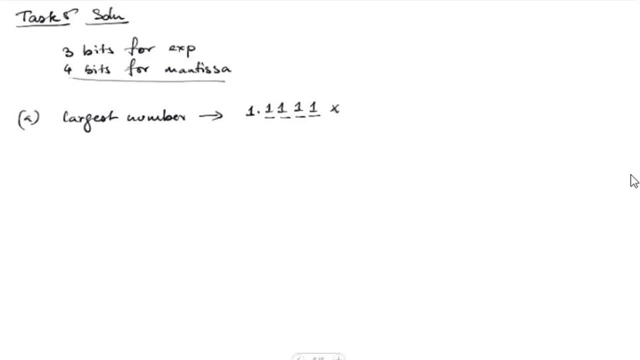 So we'll fill it up with all 1s here times, as it's the binary numbers. we have 2 to the power exponent, which is 3 bits. As said to us, we have 3 bits for the exponent. 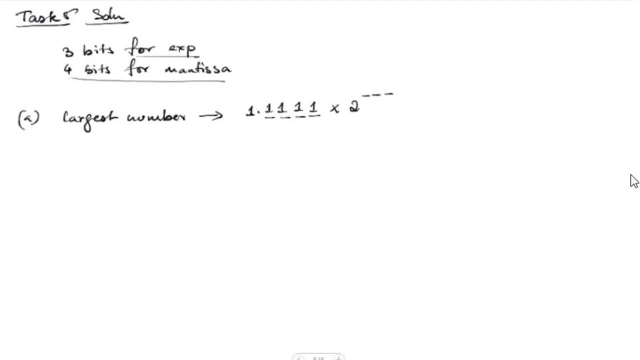 And also as we have to find out the largest number that this machine can represent. so we'll fill up all this Positions in the exponent with 1s, because that will give us the largest number, right, Okay, so we have got 1.1111 times 2 to the power 111.. 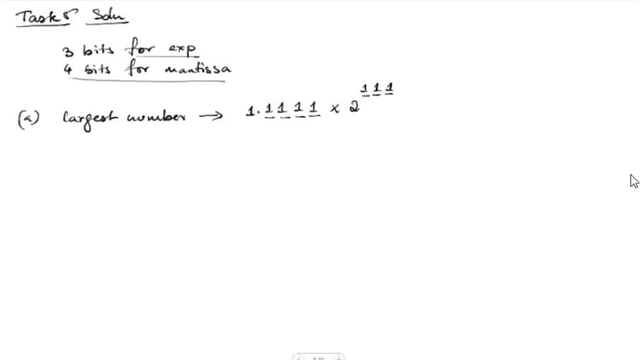 Now we have to convert this to the decimal number, So you already know the place values We have here: 0, and this one is minus 1,, minus 2,, minus 3, and minus 4.. And now we can multiply all of them. 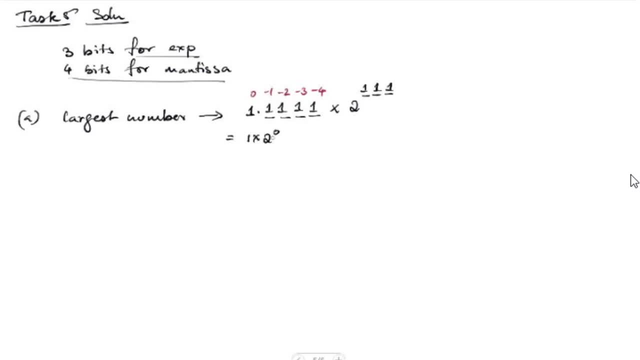 So 1 times 2 to the power 0, plus 1 times 2 to the power minus 1, plus 1 times 2 to the power minus 2, plus 1 times 2 to the power minus 3, plus 1 times 2 to the power minus 4.. 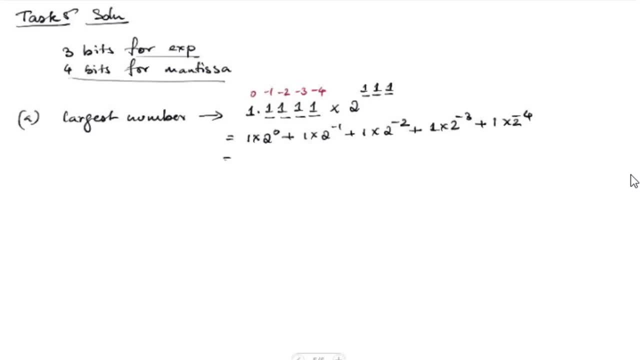 So here we have got- and we'll keep this maybe in a bracket- and times 2 to the power 111.. And if you add this all here you will get. let me write the values at first. So this is 1, plus 0.5, plus 0.25, plus. 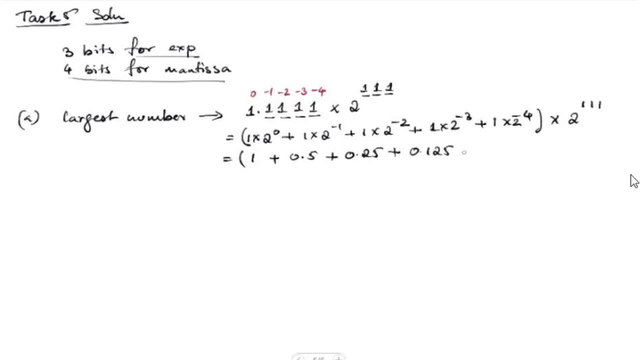 0.125, plus 0.0625, times 2 to the power 111. And this all will give us 1.9375, times 2 to the power 111.. So now let's convert this 3 ones here, or the exponent: 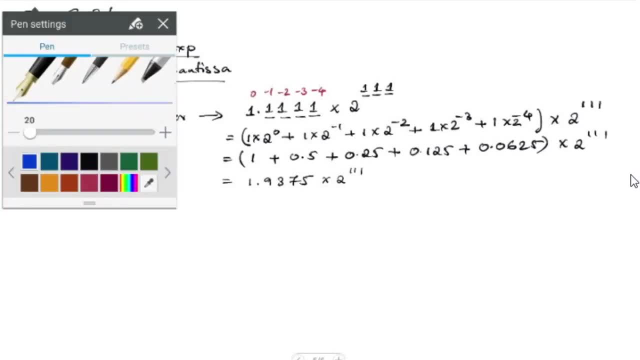 So, trying to convert the exponent, I'll do it maybe above here. So you have the 1, 1, 1 here And the place values of them is 0, 1, 2.. So you have 1 times 2 to the power 2, plus 1 times 2 to the power 1, plus 0 times 2 to the power 0. 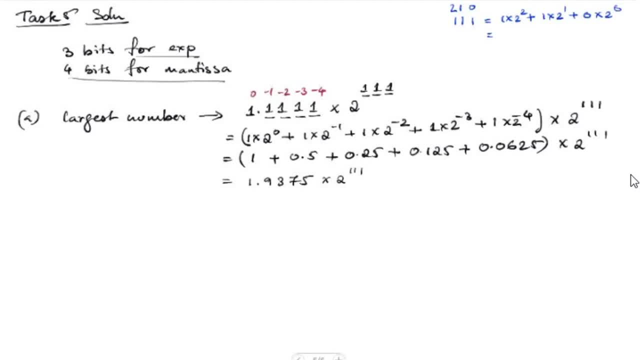 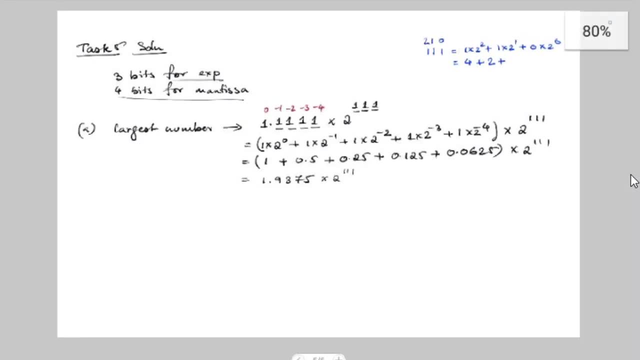 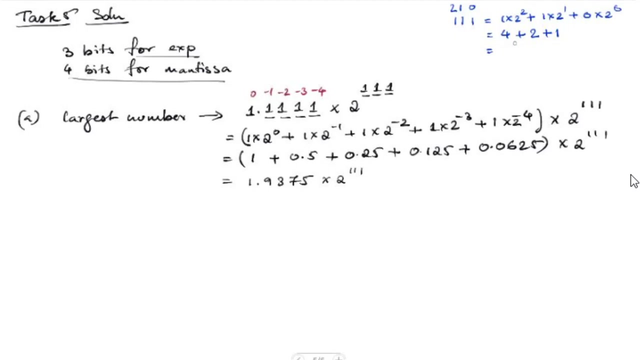 And that will give you: 2 to the power 2 is 4, plus 2 to the power 1 is 2, plus 2 to the power 0 is 1.. Which is equal to 4 plus 2 is 6, plus 1 is 7.. 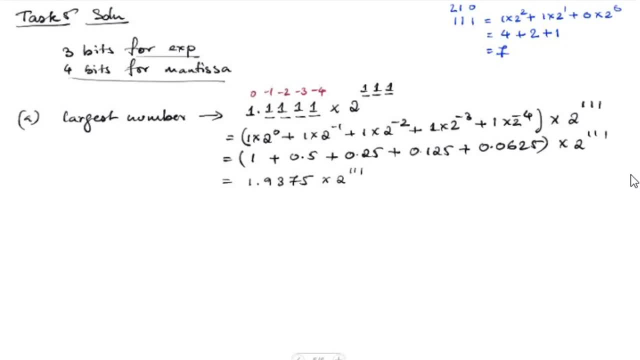 So then we have this number here. You can see it is 1.9375, times 2 to the power 2.. So you have 1 times 2 to the power 7,, which is equal to 248.. 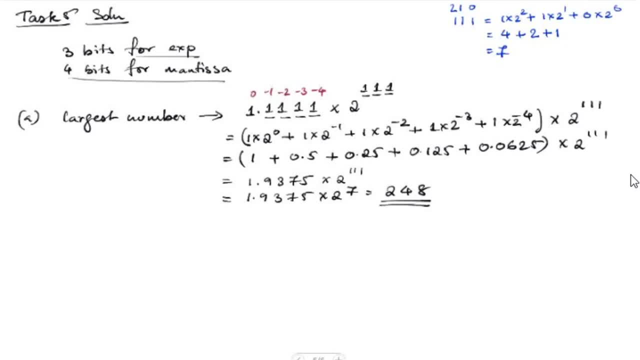 So this is the largest number that this computer can represent. Now, working on the part B, The smallest number What this computer can represent will be: Again, we'll always start with one point, And then we have 4 bits for the mantissa, times 2 to the power, 3 bits for the exponent. 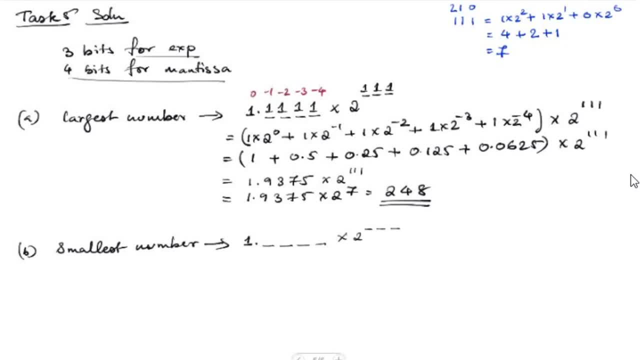 So we'll fill up the 4 bits with this time 0s, because we need the smallest possible number. So we'll fill it up with 0, 0s, 0, 0, 0.. 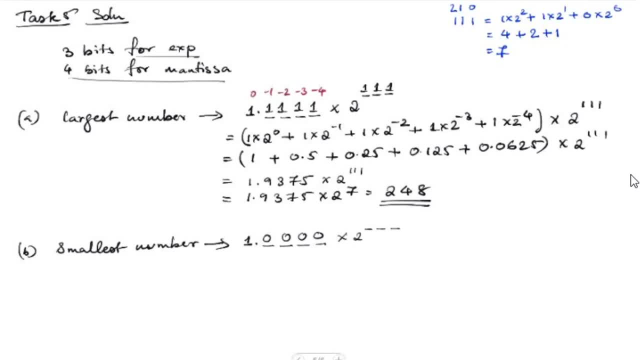 And 2 to the power, not 0s, but minus 1, 1, 1.. So we take the largest possible number and we negate it. Okay, So here now this one will be, If you convert it to the decimal we will have here. 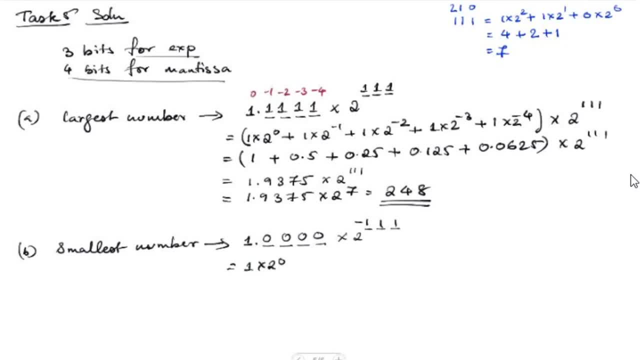 1 times 2 to the power 0. And the rest is all 0s here, so we don't need to multiply those. And times 2 to the power minus 1, 1, 1.. And, as you know, 1, 1, 1 is 7 here, so we have minus 7 this time. 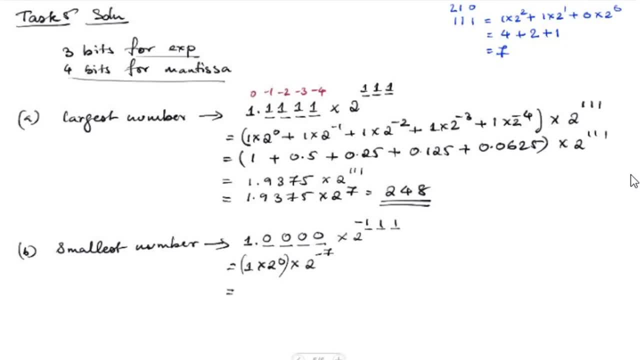 So this: So 2 to the power 0 is 1, actually, So that's 1 times 2 to the power minus 7, which is 7.8125 times 10 to the power minus 3.. 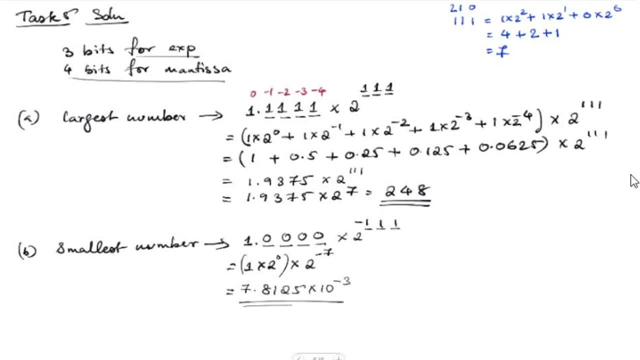 So this is the smallest number that this computer can represent.